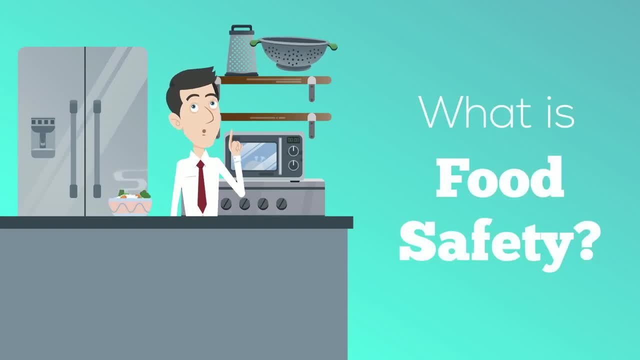 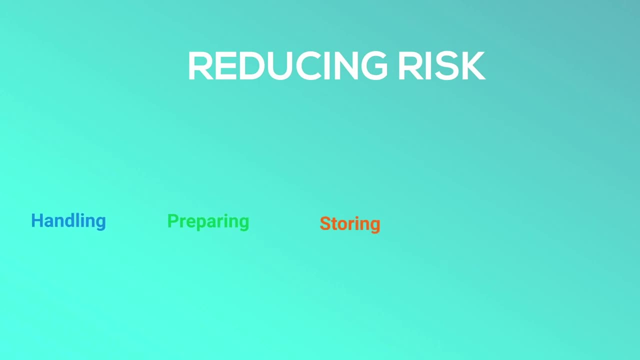 Food safety can be defined as handling, preparing and storing foods or drink in a way that best reduces the risk of consumers becoming sick from food borne disease. The principles of food safety aim to prevent food from becoming contaminated and causing food poisoning. With this in mind, ensuring that food is safe for human consumption is likely the most critical. 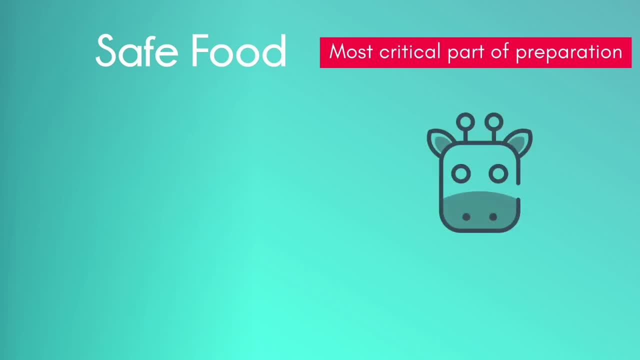 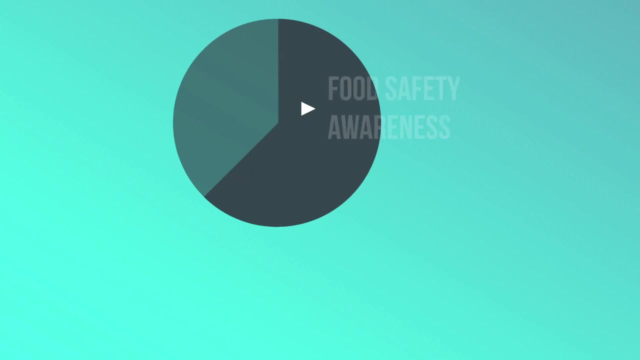 part of the food preparation process. This ranges from what is called farm to fork, meaning from the farms all the way to your plate. This means that food safety is important at home as well as in the restaurant, retail store or food factory. There has become an ever increasing awareness of food safety by the general public and news. 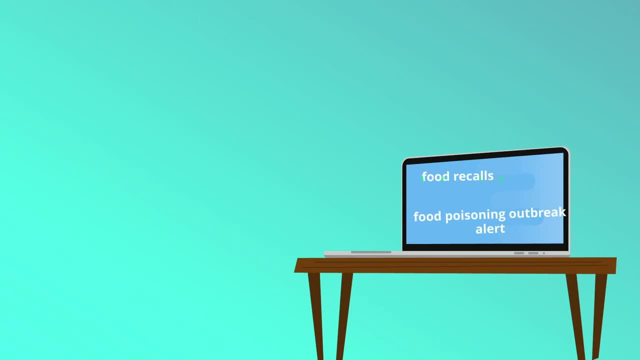 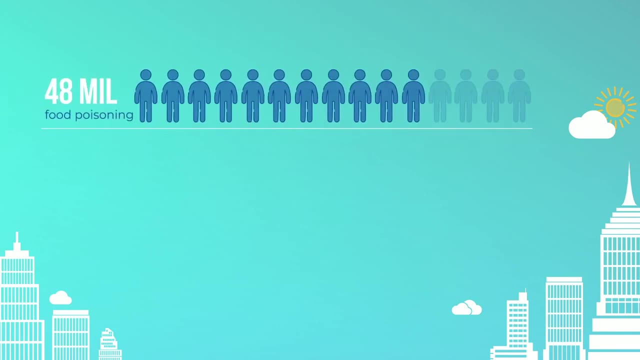 agencies are reporting on food recalls and outbreaks much more often. Reviewing the available stats, the CDC estimates that each year 48 million people get sick from a food borne illness, 128,000 are hospitalized and 3,000 die from food poisoning in the. 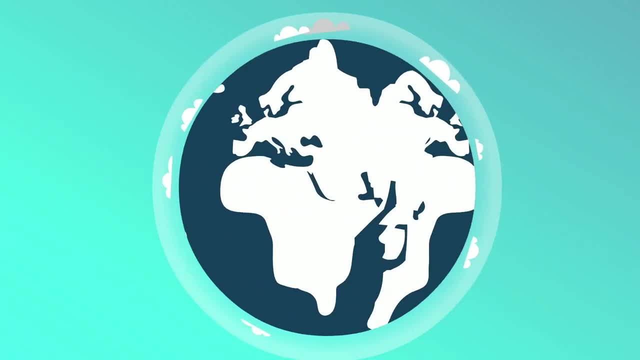 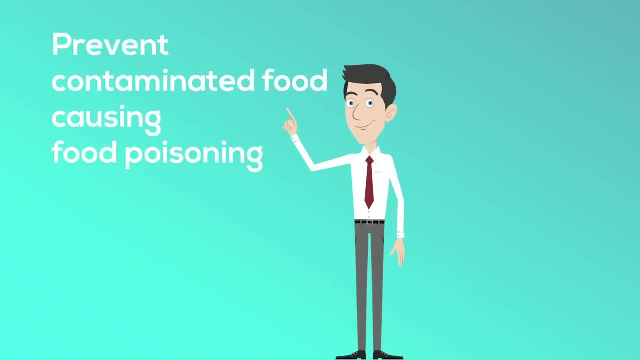 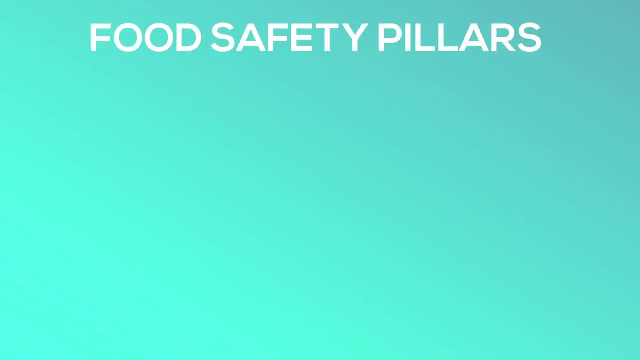 US each year. Food safety is clearly a global concern that covers a variety of different areas of everyday life. The principles of food safety aim to prevent food from becoming contaminated and causing food poisoning. Food safety can be achieved in five basic pillars: Proper cleaning and 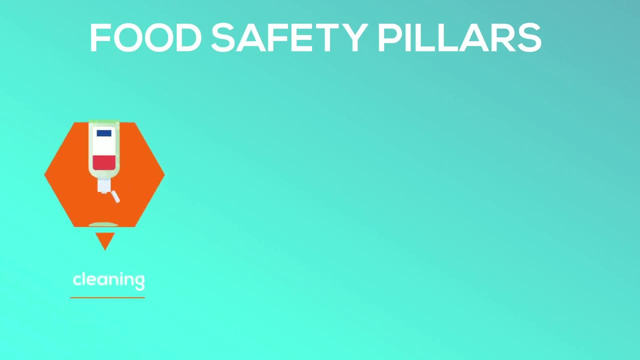 sanitizing of all surfaces, equipment and utensils. Maintaining a high level of personal hygiene, especially hand washing. Keeping foods cold when needed and keeping foods hot when required. Storing foods in a way that prevents cross contamination And cooking reheating. 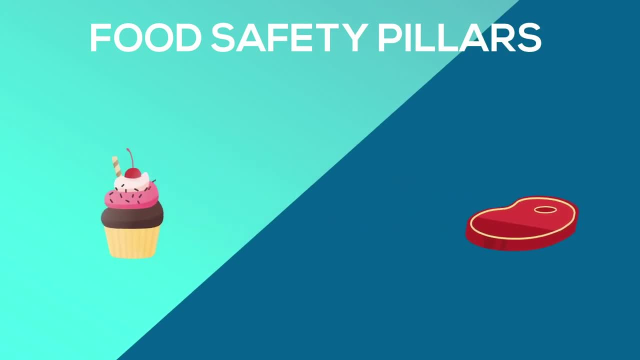 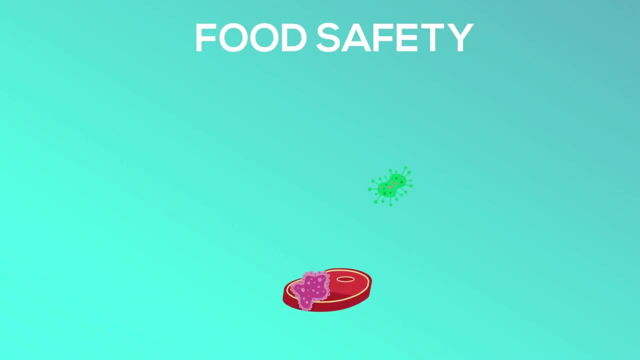 and cooling of foods, as well as the prevention of cross contamination during the preparation process. Food safety is important for the following reasons: If food or drink is not safe to eat, you cannot eat or drink. The easiest example of this is safe drinking water. You would 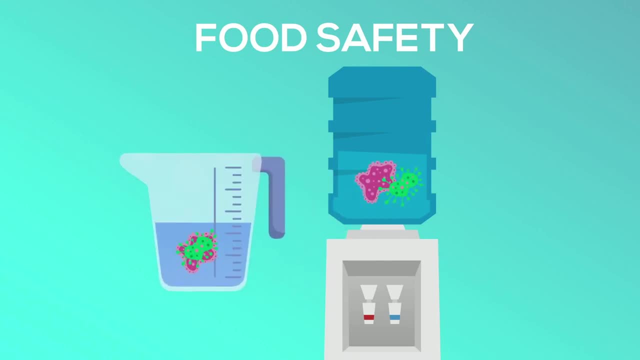 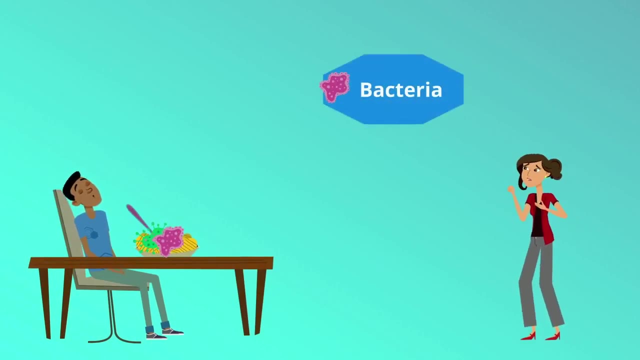 never drink water that did not come from a reputable source. The very same principle applies to food. Every day, people worldwide are being forced to eat and drink. They are being forced to eat and drink until they get sick. from food or drink, they consume Bacteria, viruses and 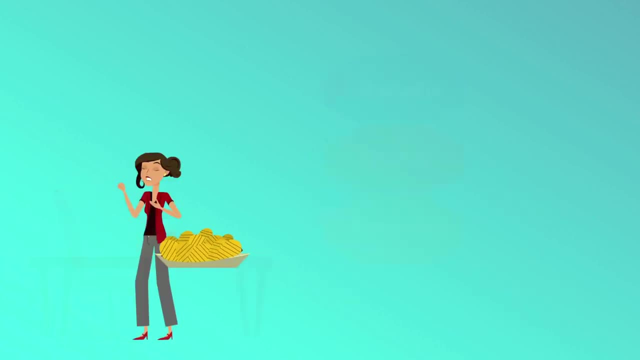 parasites found in food can cause food poisoning. There is no immediate way of telling if food is contaminated, because you cannot see it, taste it or smell anything different from the norm. Food poisoning can lead to gastroenteritis and dehydration, or even, potentially, even more.